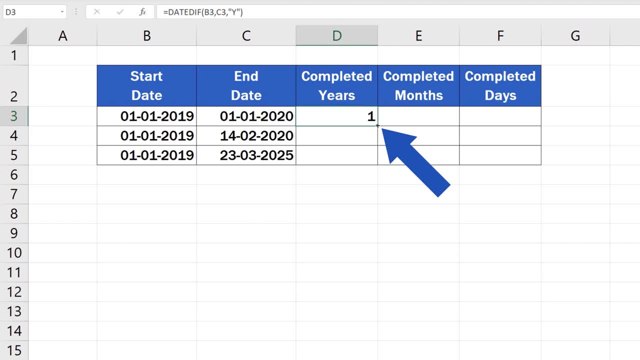 Click on the bottom right hand corner of the cell containing the formula and drag it through ALL the rows where we need the number of years calculated. Perfect Excel has calculated the number of COMPLETED YEARS that pass between the dates in each row, But we still need to calculate the number of MONTHS AND DAYS. So let's move on. 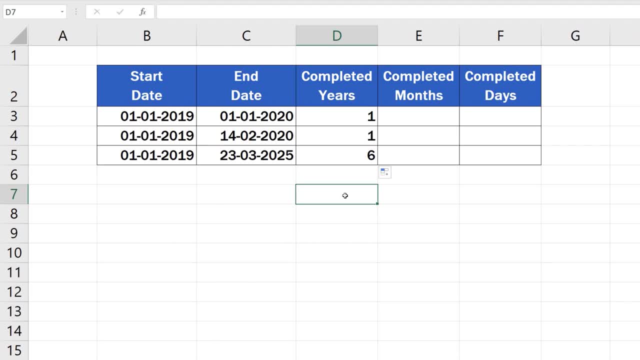 and see how many months and days pass between the two dates. We'll use the same function but we'll need it slightly amended. You'll see the following operation in the video: treatment occurs. This is the form with a warp phase of 5000.. This is an estimate of the amount of years that pass during every date. 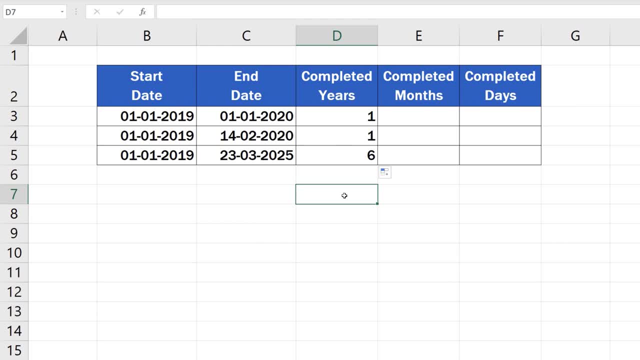 This is the little change we need to make to the formula. Click again on the target cell and follow the steps you've just seen. Type in the equal sign, then enter DATEDIF, then the start date, a comma, the end date. 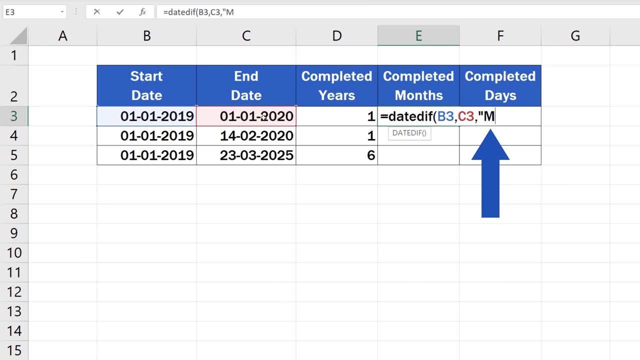 But now, instead of typing Y type M for months because we want to find out the number of completed months, Close the brackets and the result appears right in front of us in the target cell. There's no easier or quicker way to calculate the accurate number of months passed between. 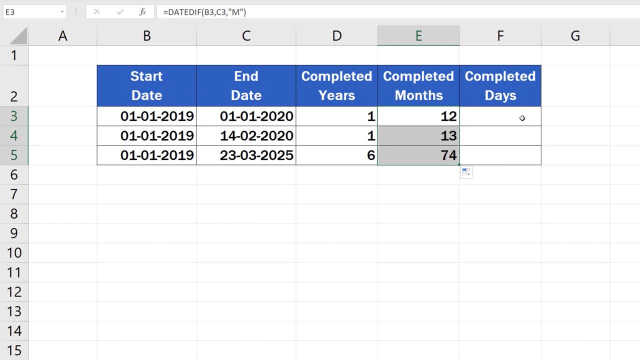 two dates And what do you think comes in the formula to calculate the number of completed days? You're about to find out whether you guessed right. Start as usual, type in the equal sign: dateDIF: start date and end date all separated with: 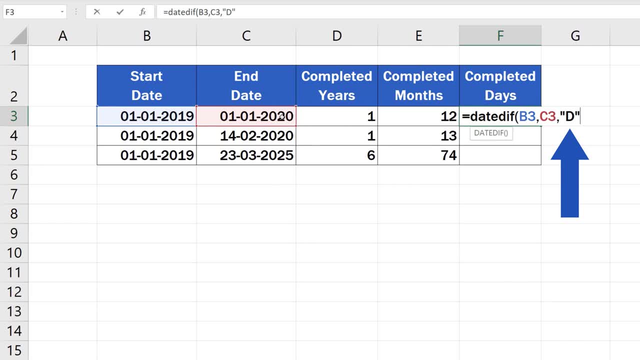 a comma. And now we'll finish the formula with D for days. Close the brackets, hit enter. The number of completed days is as easy to figure out. It's the number of completed months or years. This is a universal way to calculate the difference between two dates working within any time. 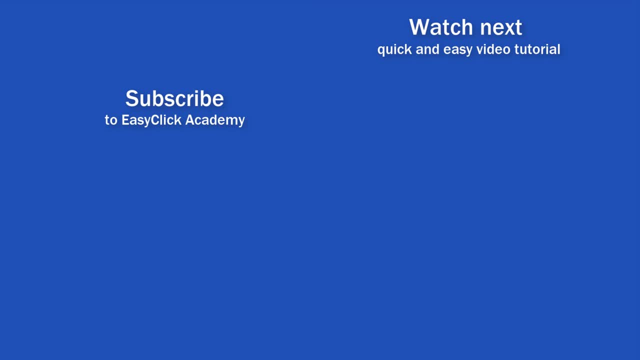 data in a table. If you found this tutorial helpful, give us a like and watch another video tutorial by EasyClick Academy: Learn how to use Excel in a quick and easy way. Is this your first time on EasyClick? We'll be more than happy to welcome you in our online community. 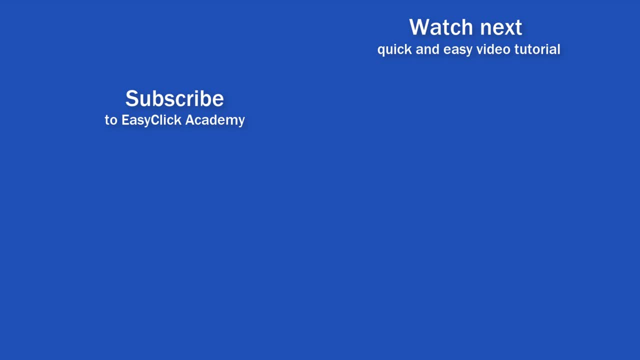 Hit that subscribe button and join the EasyClickers. Thanks for watching and I'll see you in the next video.